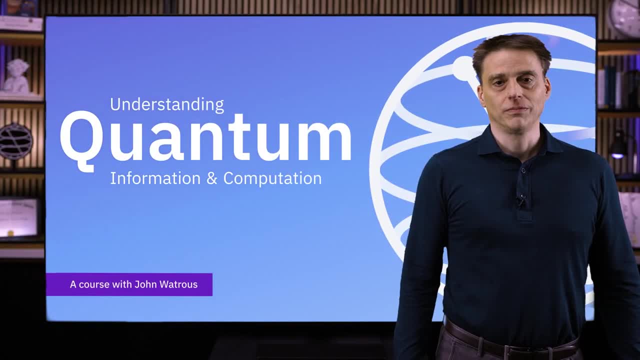 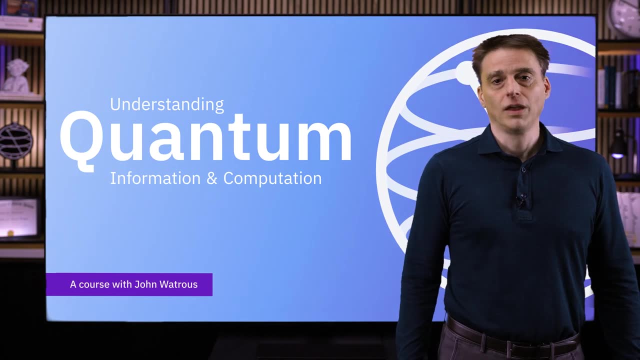 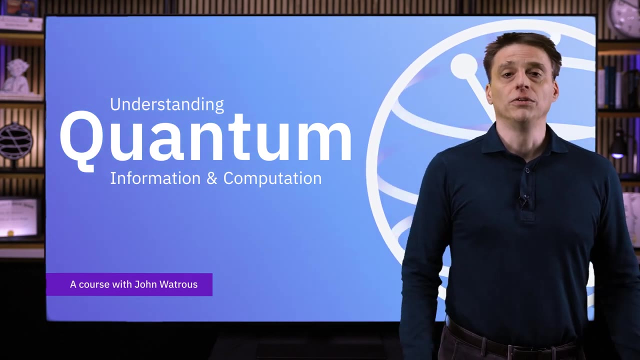 Hello and welcome to Understanding Quantum Information and Computation. This is a series that explains how quantum information and computation work at a detailed mathematical level. It's meant for anyone that wants to learn about quantum computing at a level that's comparable to what's taught in universities around the world to students at the advanced 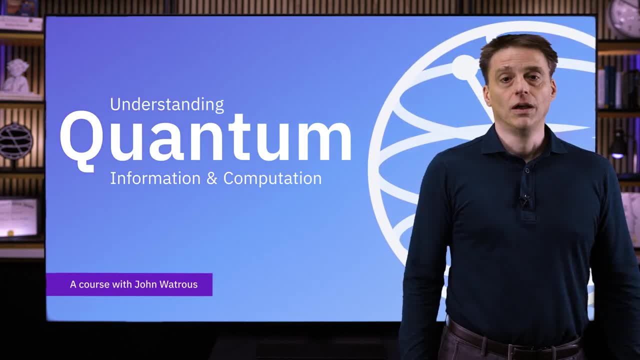 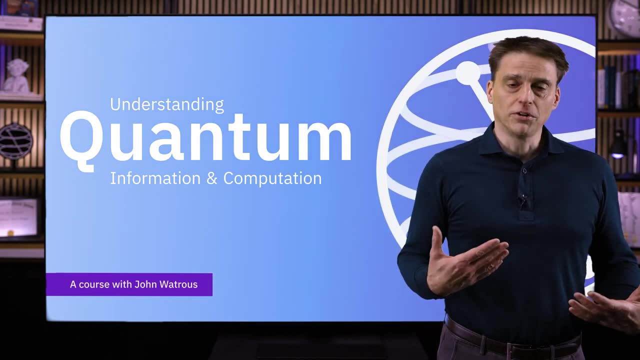 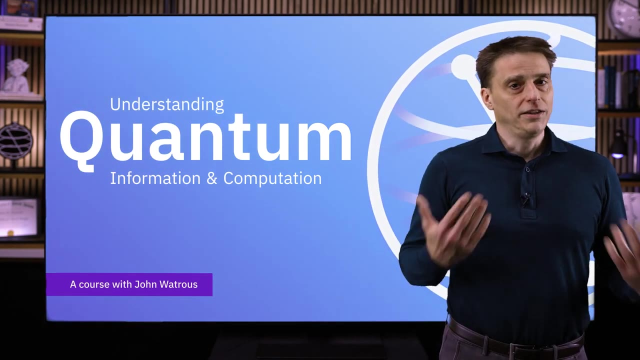 undergraduate or introductory graduate level. My name is John Watrous and I'm the Technical Director of Education at IBM Quantum. I first learned about quantum computing in 1994 and I've been studying, researching and teaching it ever since then. The idea behind this series is pretty simple. 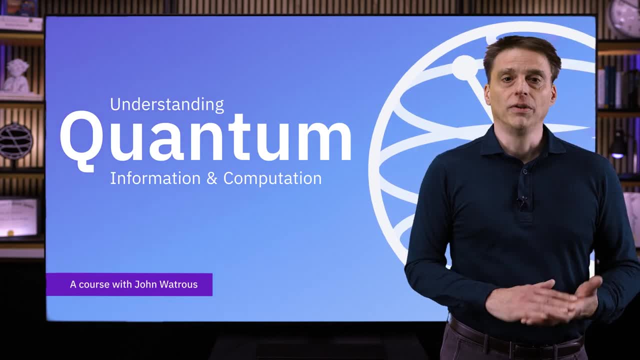 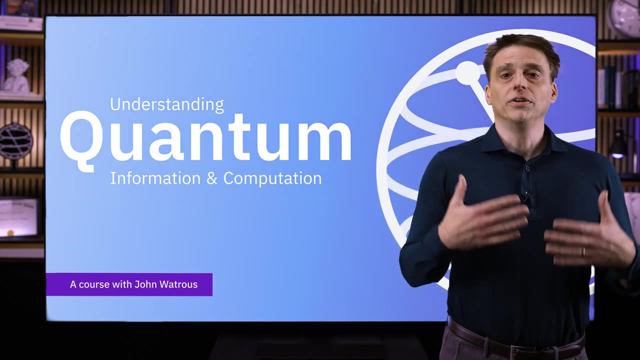 There are a lot of people all around the world that want to learn about quantum computing and, ultimately, to make contributions of their own to its development and its usage. My goal for this series is to make this content available to anyone that wishes to make use of it. 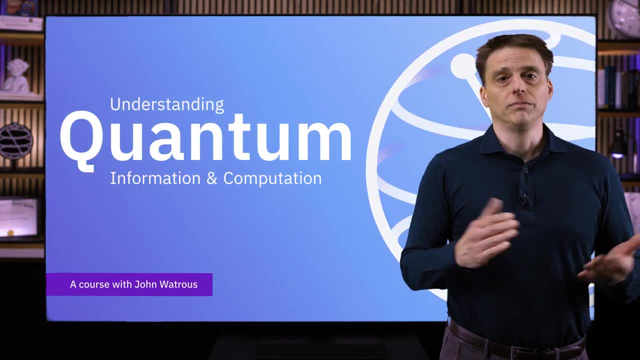 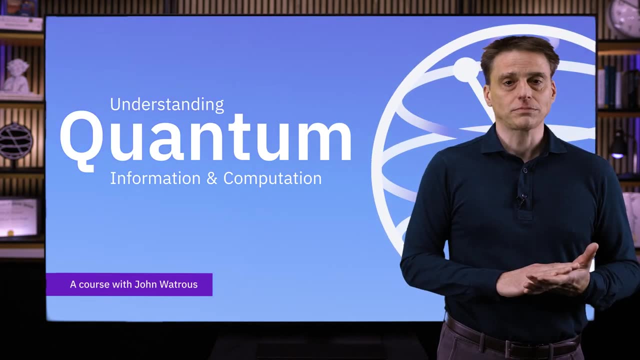 Now, the series surely won't have value for everyone. If you're not interested in learning more about quantum computing and quantum computing, or if you're interested in getting into the details and learning about the mathematics behind quantum computing, it probably won't appeal to you. 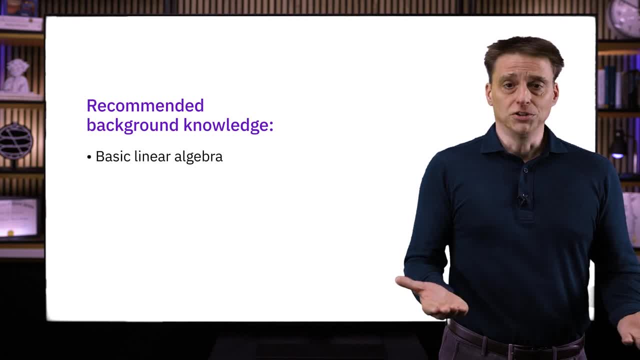 To follow these videos, you'll need to understand the basics of linear algebra, including vectors and matrices, and how to work with them, as well as notions such as linear independence, bases and dimension. You also need to understand how complex numbers work and you need to be comfortable with. 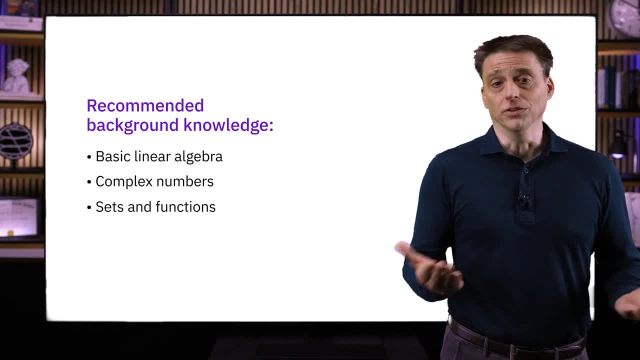 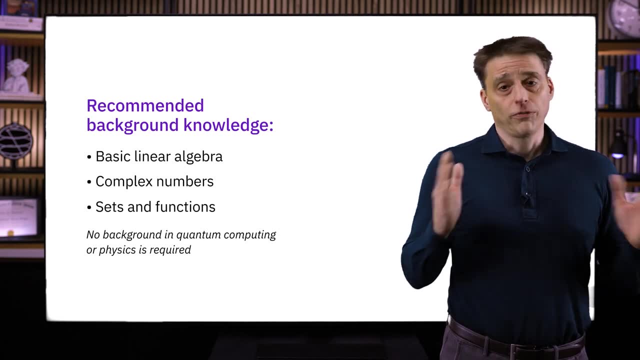 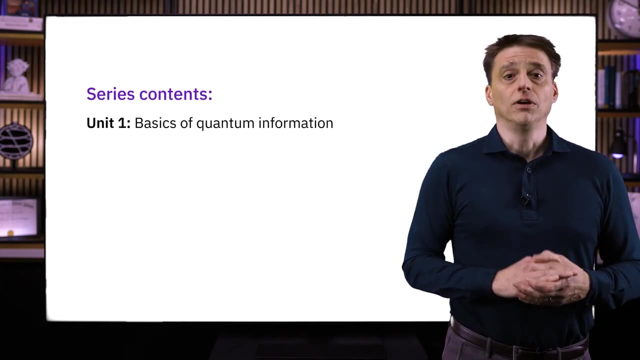 some basic mathematical concepts such as sets and functions. There's no expectation that you have any background in quantum computing, quantum mechanics or physics in general. Unit 1 of the series explains the basics of quantum information, including quantum states, measurements and operations, how quantum circuits work and some important examples, such as. 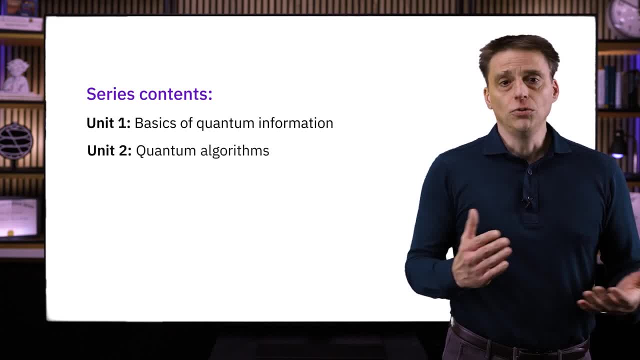 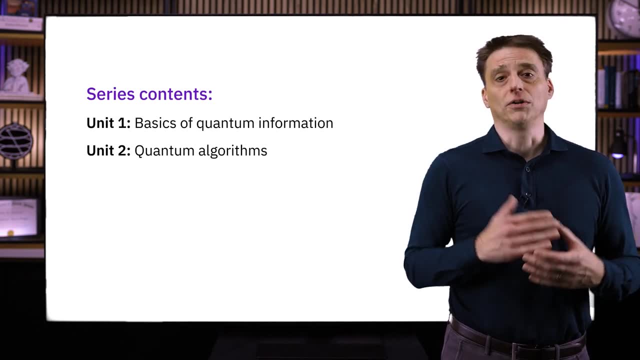 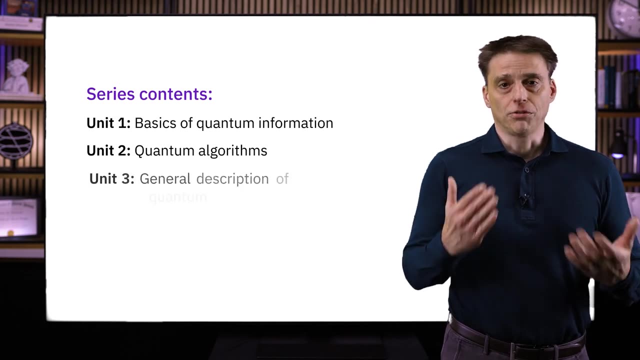 quantum teleportation. In Unit 2, we'll explore quantum algorithms, including Shor's algorithm for factoring integers, as well as some algorithms that are better suited to the quantum devices that are available to us today. In Unit 3, we'll dive a bit deeper into quantum information and we'll talk about how it can.